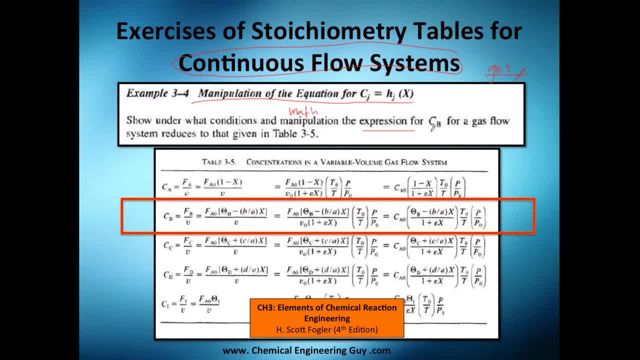 what kind of math do you use for the expression of concentration of B for a gas flow system that reduces to that given in table 3-5.. So first of all, we're looking for concentration of B, which is this one, this here and this here, which is the same as this one, which. 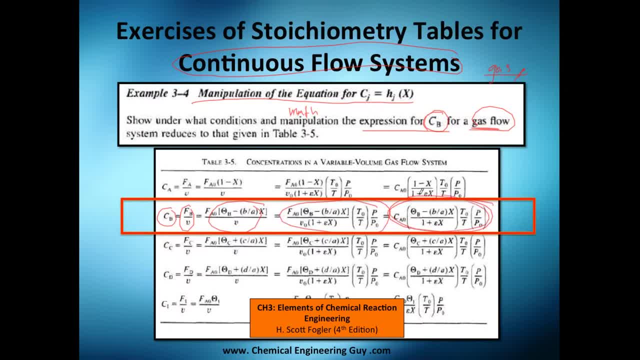 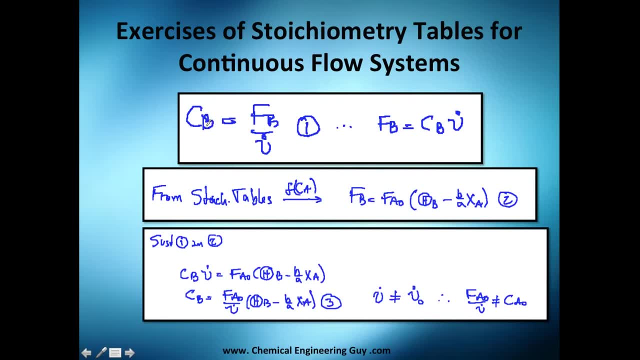 is the same as this one. So how do we get this value? That's what they are asking us, So let's do it First thing. first remember that concentration of B at any moment is flow of B divided by volumetric flow rate. Or if we send this one multiplying, we get flow of B equals this here. 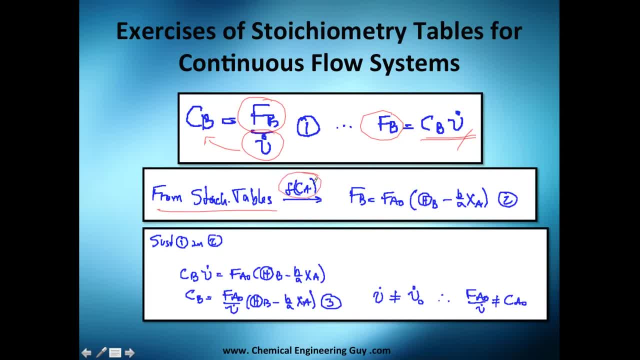 Now from stoichiometric tables. remember that that's in function of concentration. we can change it. We change: flow of B equals initial flow rate. Flow rate of A, this fancy function. since it's a reactant, it's negative and this stoichiometric. 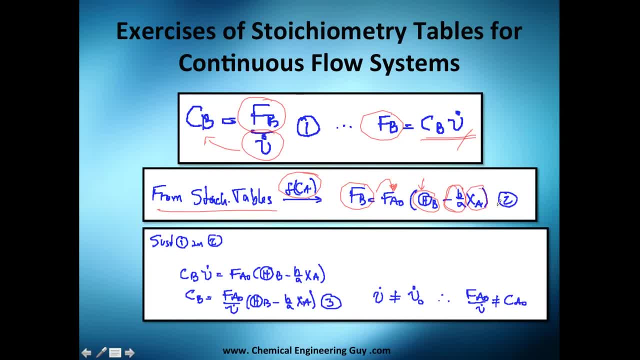 value B divided by A times the conversion. Now let's suppose you have this one- this is equation number one- into we got concentration of B times volumetric flow rate, which is: this part equals F of B And this is F of. 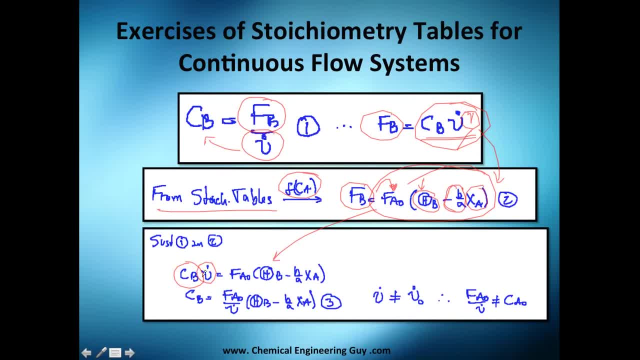 B. So let's put this F of B here And send away this again. And one thing first: probably you want to force this to be concentration of A, but it is not, because this is not an initial value. So because it is not an initial value, you know that F of A at the initial is not the 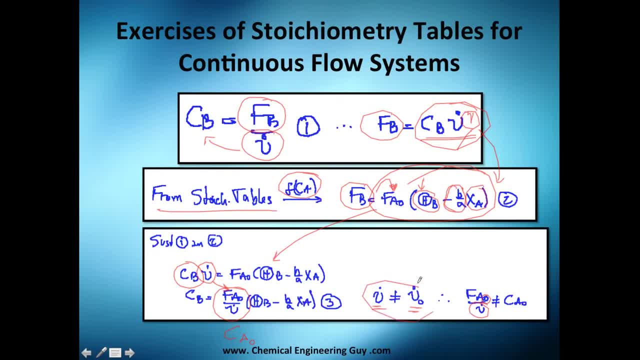 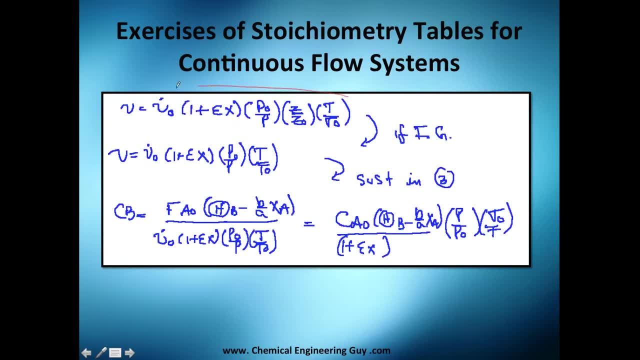 same as this here, Because they are not the same, So we cannot say it's concentration. Actually, we will need to find out this volume equation. hopefully you remember it. It's the pressure changes, The C changes, The temperature changes And the volume change here. 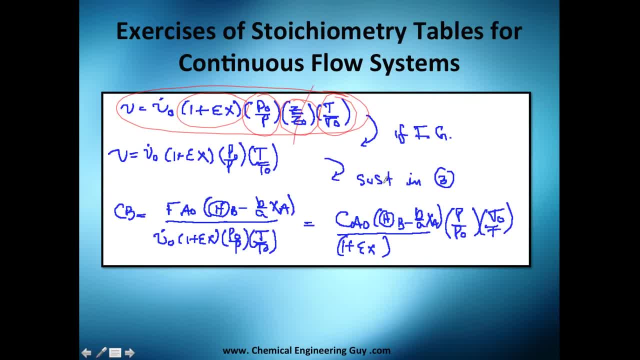 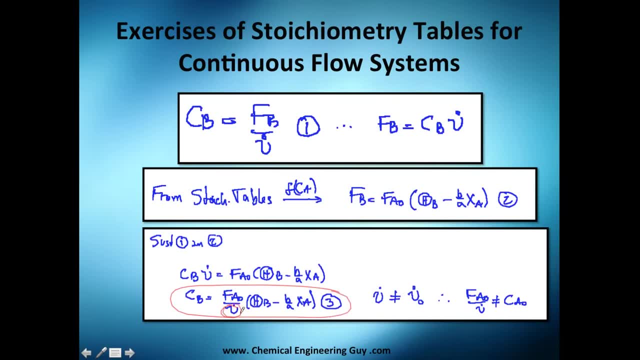 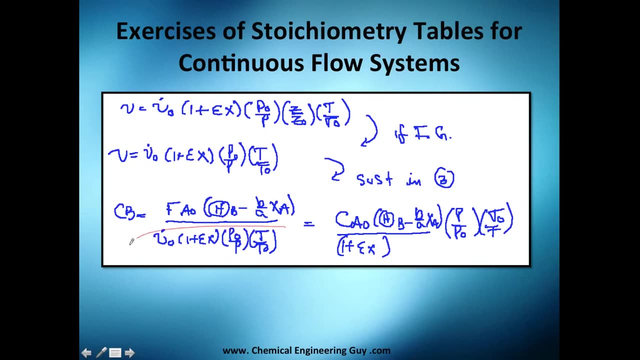 Now, if ideal gas, take away that C and substitute this in equation number three, which is here, Right here. So we want to substitute the values here And we got this. This huge equation is down and this stays the same here up. 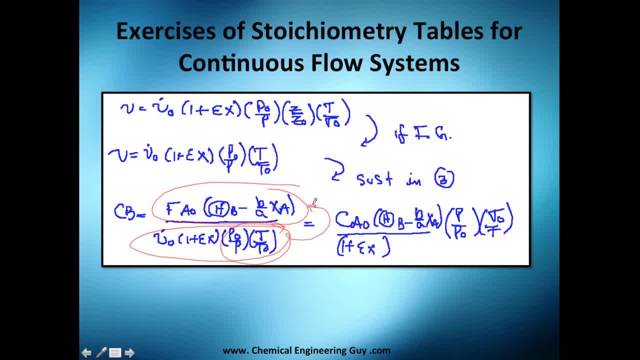 Now I want to change these up, Take them all up here, And this time we can do this, We can force the concentration because both are initials. So this is concentration of my initial value, Because we have initial here and initial here. 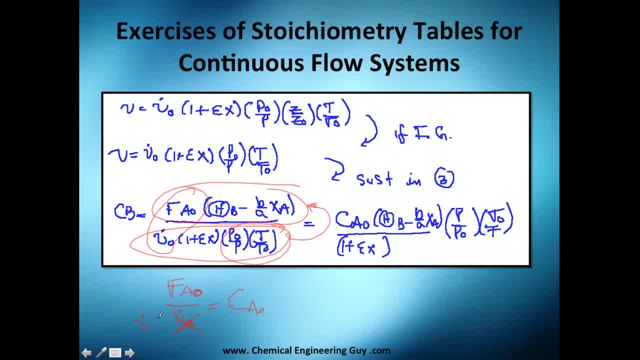 Before we couldn't do that because this was not the initial value, This was the volumetric flow rate at any moment or at that conversion. But right now we can do it. So this is the concentration We got here. Now this stays exactly the same here. 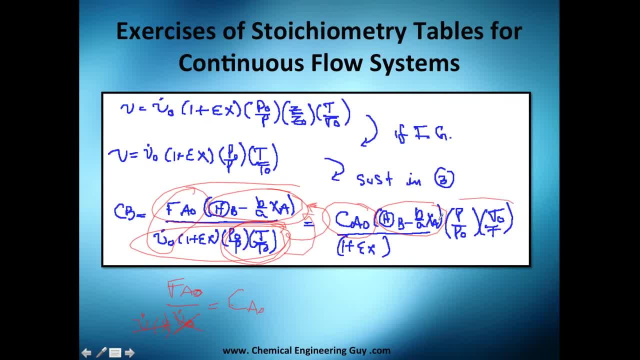 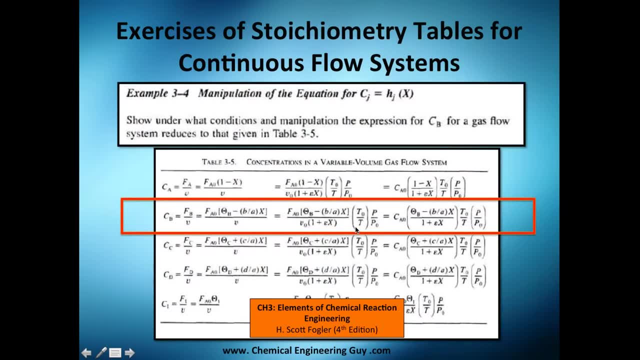 I just change this from here to here And I stay here with this value here, Which is the value they wanted me to prove Here: The temperature and pressure changes, This value, the concentration I told you about, and this right here. 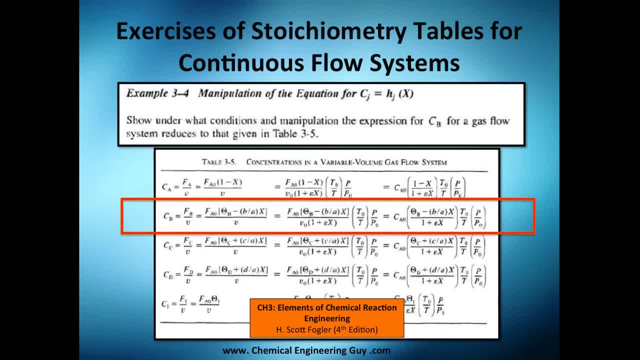 And that's how you get them, guys. It was so easy. this example, I like it. I like it because it helps you to work out with these numbers And, at the same time, it's good for you because you get to use the table. 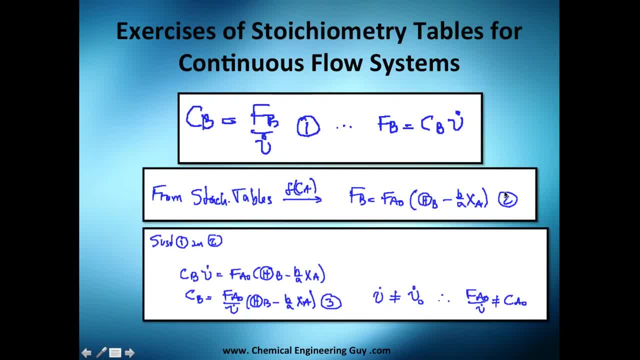 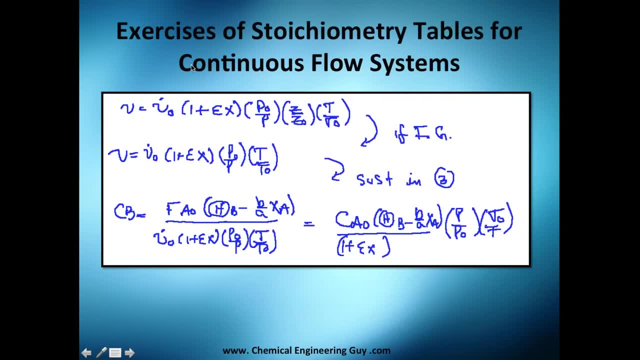 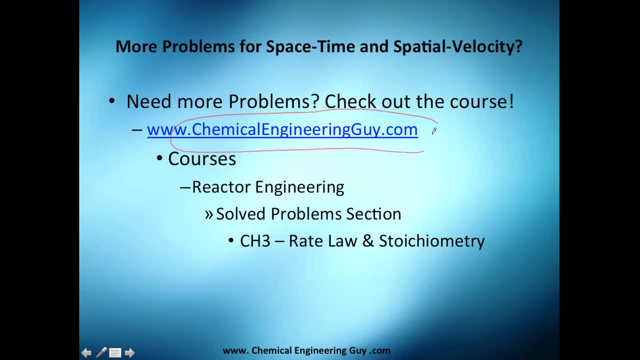 I told you I didn't like it much, But we use it And that's everything actually. If you want more problems, we can check them out here. Go to this web page here And go to Courses: Reactor Engineering- Solve Problems. 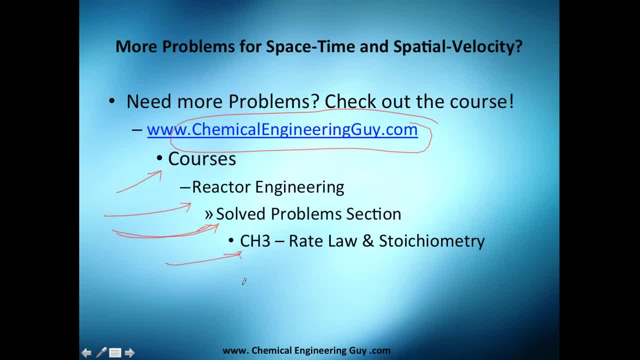 I got some Solve Problems there. Check it out And go to Chapter 3, Rate Loss. I got Problems in Rate Loss And Stereometry, How to apply all those tables. And yeah, guys, Let me cut this and check it out. 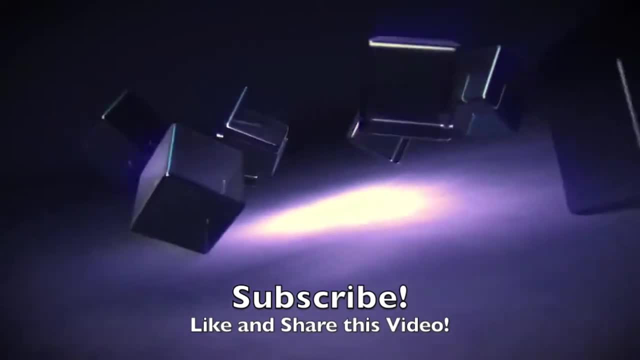 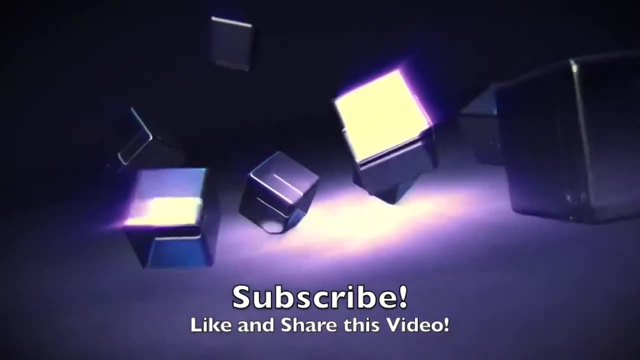 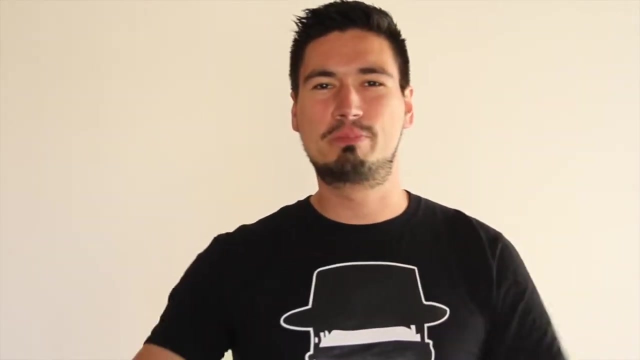 What's up guys? It's me Kevin, And I'm going to show you how to do this. Okay, Let's go. I'm a chemical engineering guy, So if you like the video, why not push the like button? It really helps me to know if you're liking the videos or if I should be changing something.